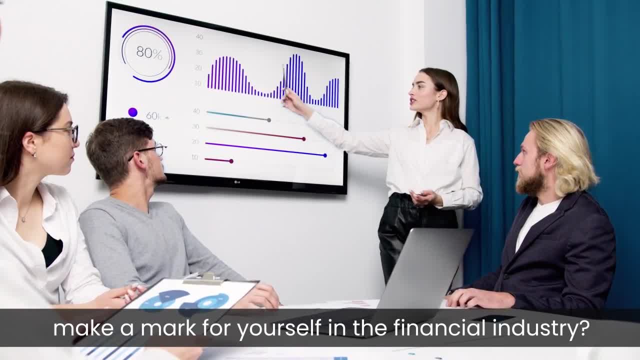 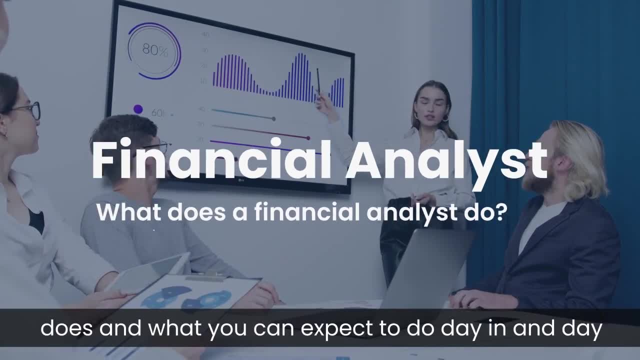 Are you looking to become a financial analyst and make a mark for yourself in the financial industry? Well then, you have come to the right place. In this video, I will tell you what a financial analyst does and what you can expect to do day in and day out, if you. 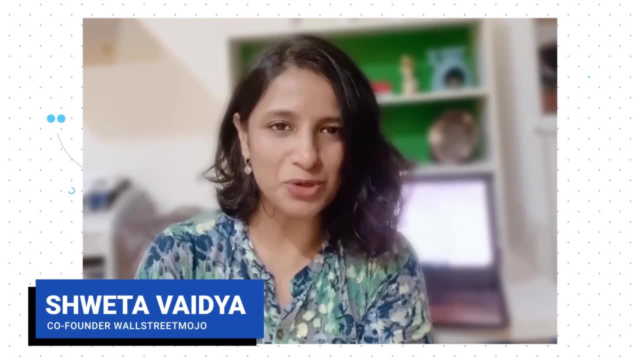 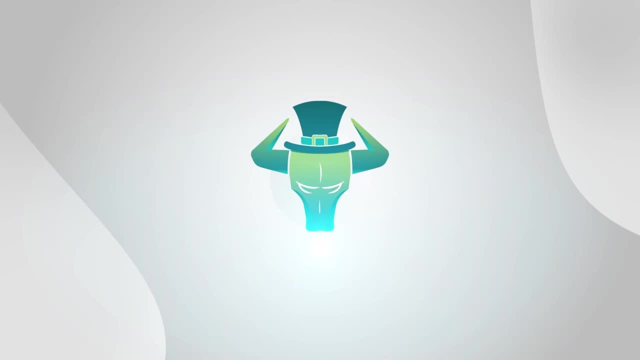 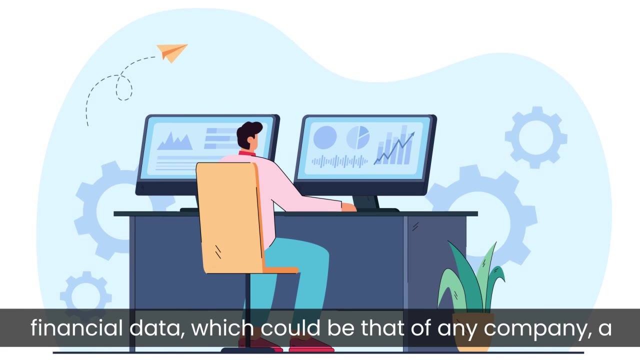 decide to become one. Hello guys, this is Shweta and welcome to the world of WallStreetMojo. In a nutshell, a financial analyst would analyze some financial data, which could be that of any company, a sector or the economy. Now they would do this to arrive at a conclusion. 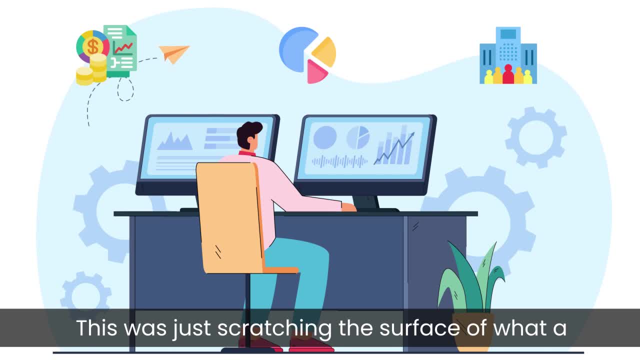 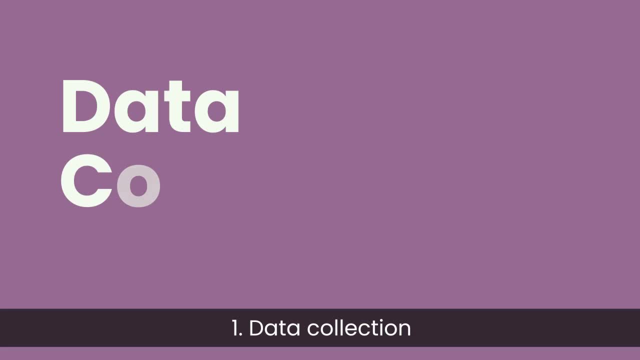 mainly to decide investment decisions. This was just scratching the surface of what a financial analyst does. Let's understand their work a bit more elaborately. 1. Data Collection. I told you right, financial analysts perform some analysis on a particular data, So the 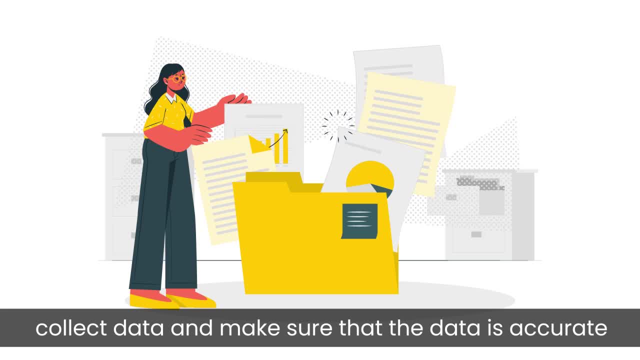 first thing a financial analyst would do is to collect data and make sure that the data is accurate and credible. Data can be collected from the company's 10K annual report, from financial websites like Bloomberg and even from the archives of the financial exchanges. 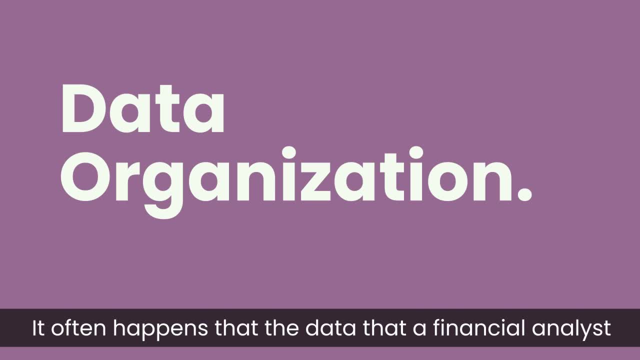 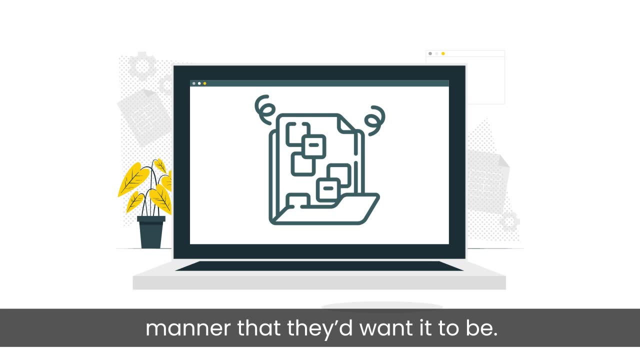 2. Data Organization. It often happens that the data that a financial analyst collects is not the same as the data that a financial analyst collects, So the data that a financial analyst collects is unorganized and not in a structured manner that they would want it to be. Financial analysts would then work to put the data in order and in a 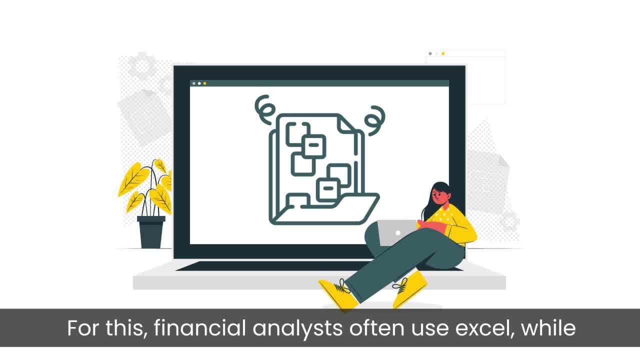 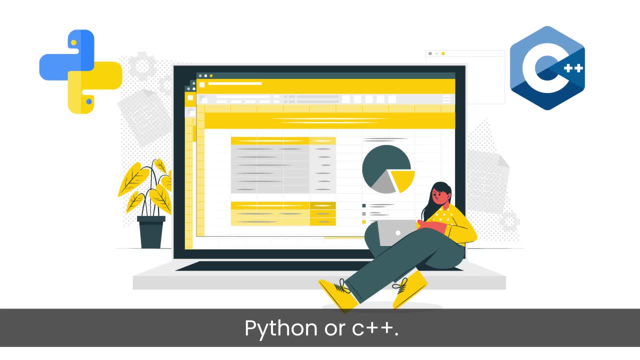 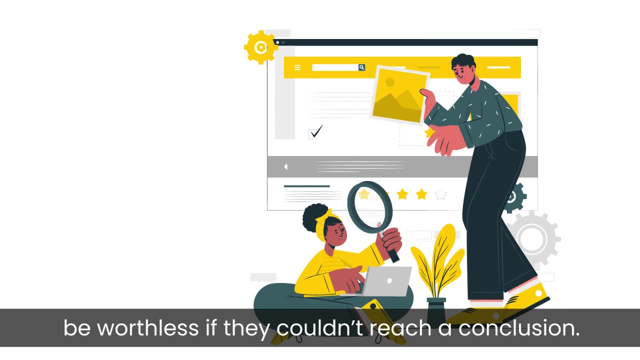 manner that would make their further work easier. For this, financial analysts often use Excel, while some may even use programming languages like Python or C++. 3. Forecasting The entire work that a financial analyst does would be worthless if they couldn't reach a conclusion. To help them with that. they would need to do a lot of work. For example, 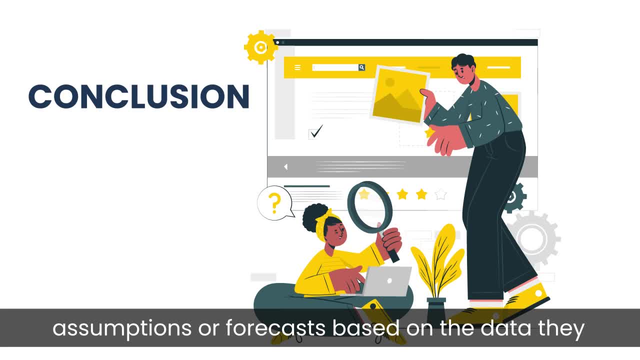 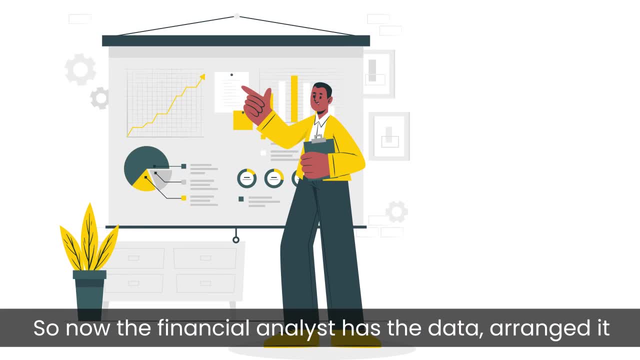 they would make some assumptions or forecasts based on the data they have. 4. Building Financial Models. So now the financial analyst has the data, arranged it properly and made some forecasts. This is a critical point. At this stage, the company's financial statements are forecasted. 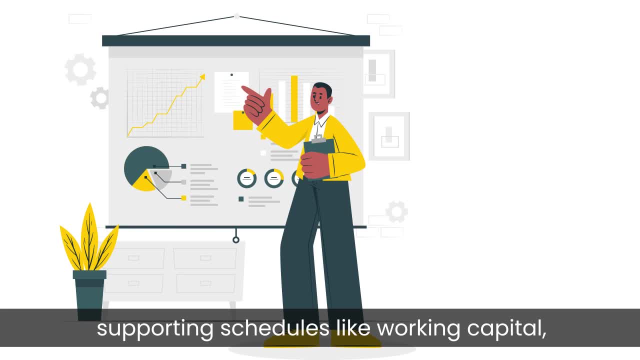 for the next 5-10 years by preparing supporting schedules like working capital depreciation schedule, shareholders' equity schedule, debt schedule and so on. Financial model building is the bread and butter of a financial analyst. Some of the common financial models are the discounted cash flow model, leverage, buyout model, mergers. 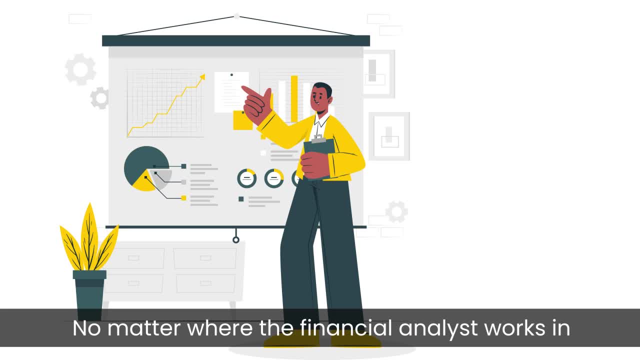 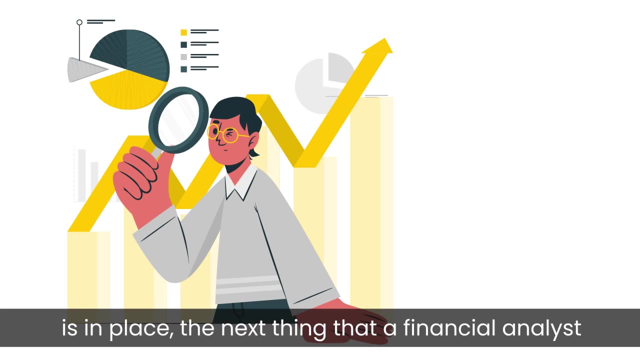 and acquisition models, etc. No matter where the financial analyst works- in investment, backing, corporate finance or even equity research- financial models will be used everywhere. 5. Analyzing Financial Results. Once the financial models are ready and everything is in place, the next thing that a financial 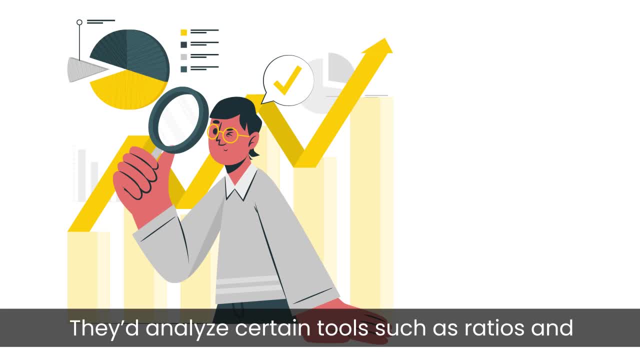 analyst would do is to analyze everything. They would analyze certain tools such as ratios and matrices, including gross profit margin, net profit margin, cost to sales ratio, debt equity ratio, etc. There are many things that financial analysts may look at to improve. 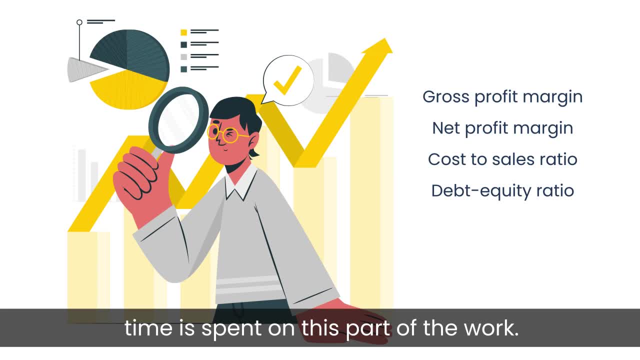 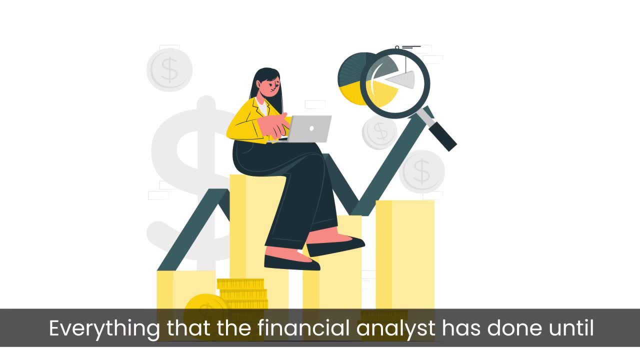 their decisions. Hence, a lot of time is spent on this part of the work. 6. Providing Recommendations Using Valuation. We are now in the end game here. Everything that the financial analyst has done until now leads them to make a conclusion and provide recommendations to the investors. 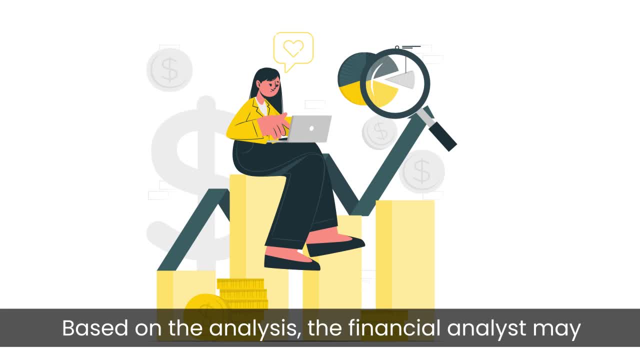 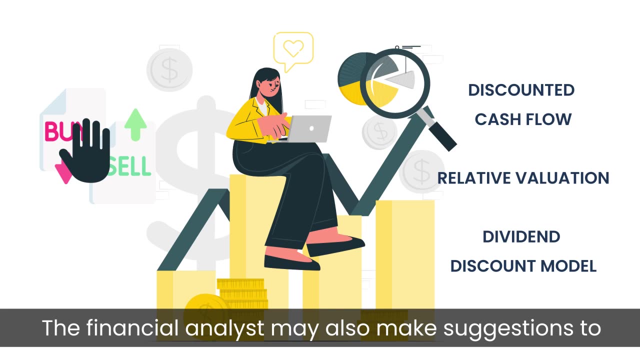 or their clients. Based on the analysis, the financial analyst may suggest investors to buy, sell or hold the stocks. This is done using various valuation approaches, like discounted cash flow, relative valuation, dividend discount model, etc. The financial analyst may also make suggestions to businesses on how to reduce costs, tap into new markets, increase efficiency. 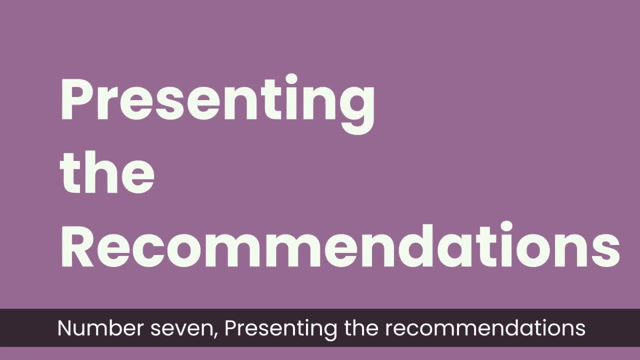 increase capital, etc, etc. But most of the time the financial analyst will only make up for what he has already done. The first step is to build financial models and plan changes etc. number seven, presenting the recommendations. it is often said that it's fine if a person is. 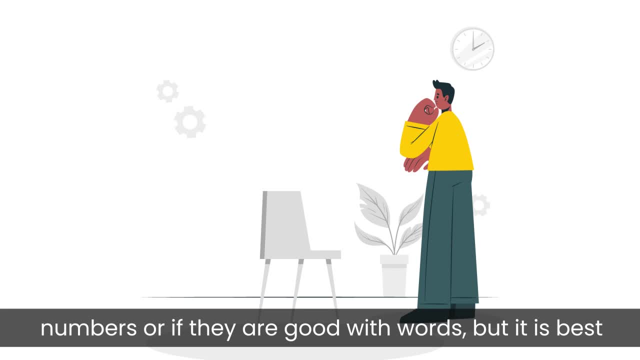 good with numbers, or if they are good with words, but it is best when they are good with both. everything that a financial analyst does involves numbers and jargons that not everyone can understand. that's why financial analysts have to present their work in an easy to understand manner.